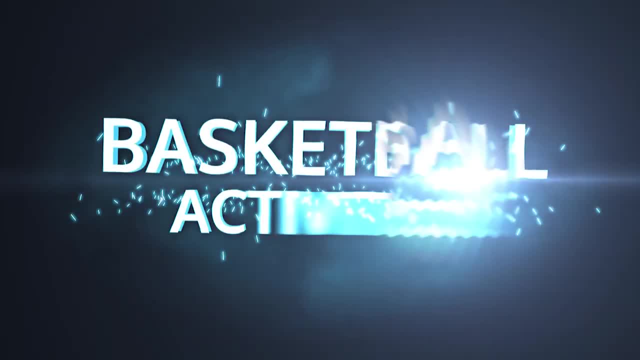 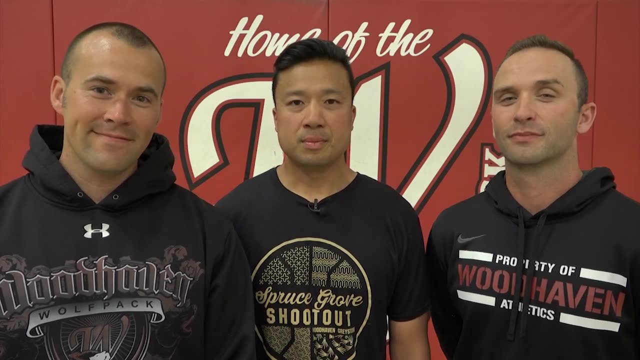 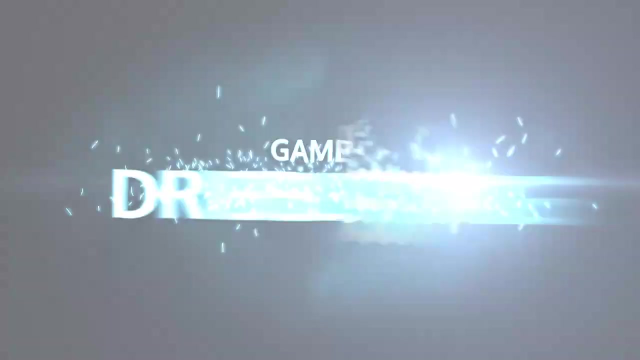 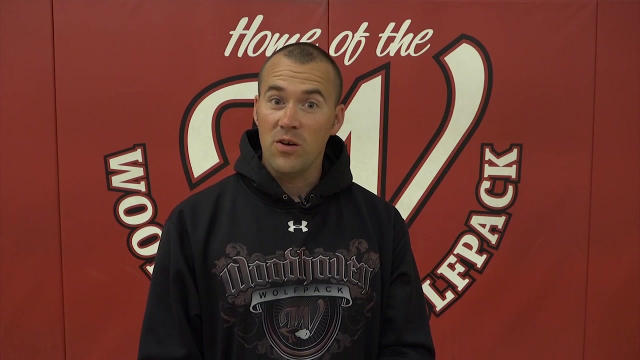 Hi. I'm Mark Bradshaw, I'm Nathan McLaughlin, I'm Will Chan and we're physical education specialists at Woodhaven Middle School, and we're here to share with you some basketball activities. The first basketball game we're going to show you is called Dribble Tag. 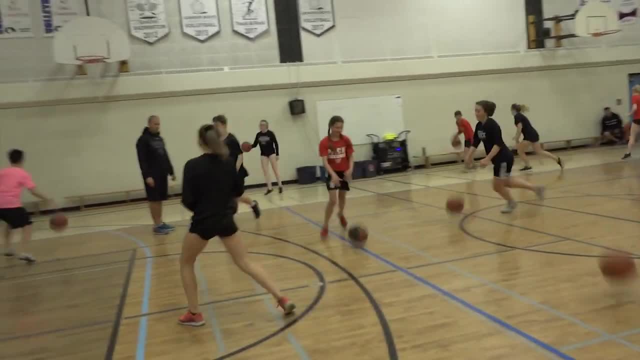 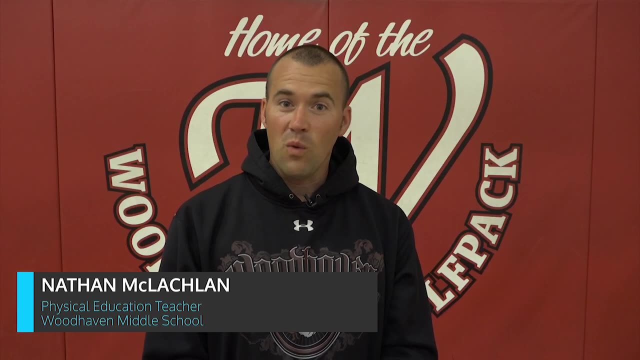 This game can be played from students in grades three and up, and it can be between 10 all the way to. we've had up to 80 kids play the game. In order to play Dribble Tag, you need one basketball per player, So if you have a large group, you're going to have to have a lot of 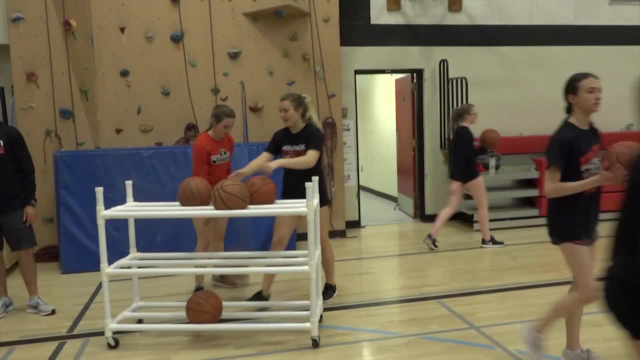 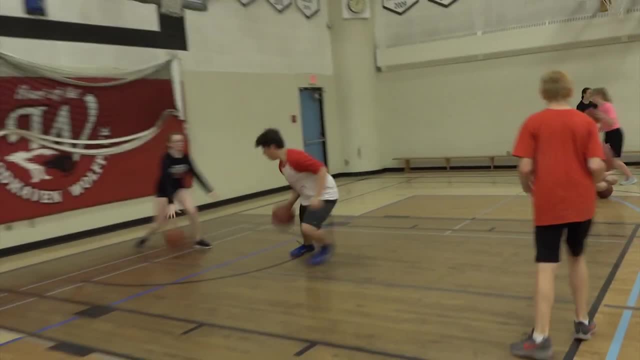 basketballs. If you have a smaller group, you can get away having a small amount of basketballs. So in Dribble Tag everybody has a basketball. You can go anywhere in the gym. Okay, there's no restrictions for space. The objective, like I said, keep your dribble alive. 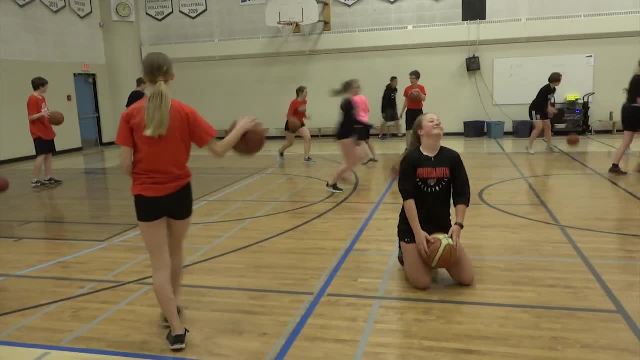 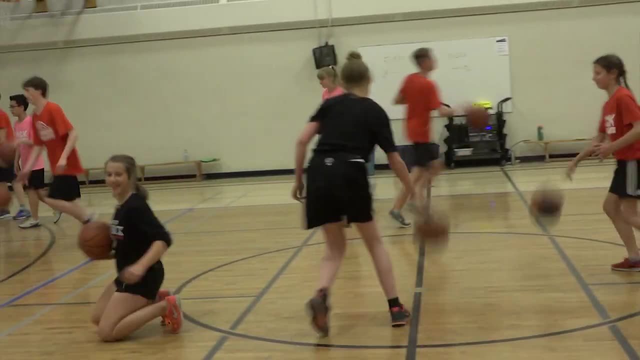 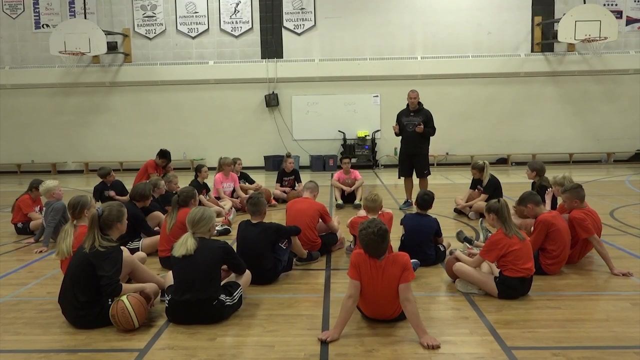 If somebody tags you, you sit down where you got tagged. How do you get back in the game when you've been tagged, When the person who tagged you is tagged by somebody else, or if we yell jailbreak or resurrection. So, for example, Austin, can you stand up, Alex can you stand up? 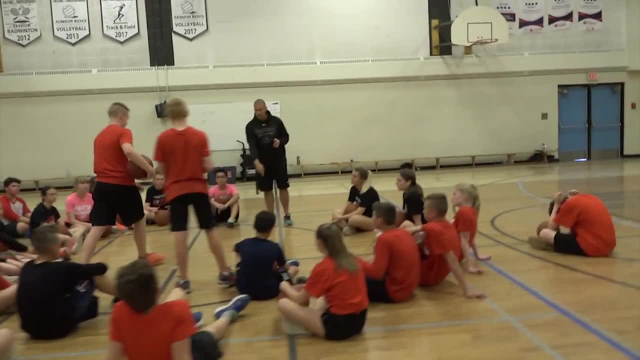 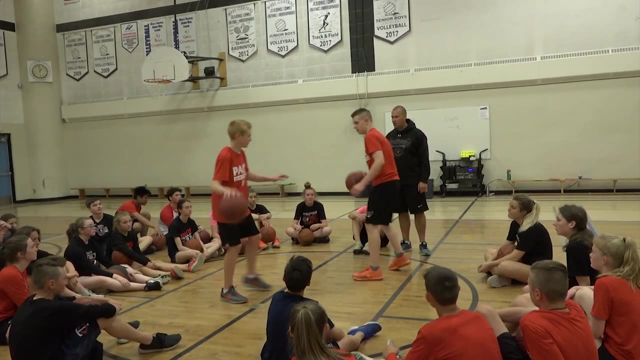 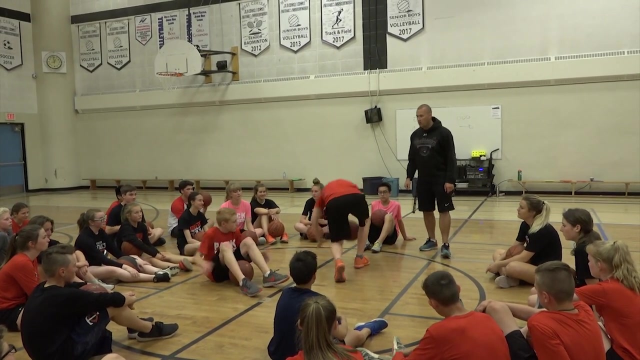 So say, these two guys are in the game, Alex over here, So they're dribbling the basketball, Dribbling the basketball. Go ahead, guys. They're going to go into tags. Alex tags Austin. Austin's going to sit down. I come along and I tag Alex. He sits down. Austin gets back up in the game. 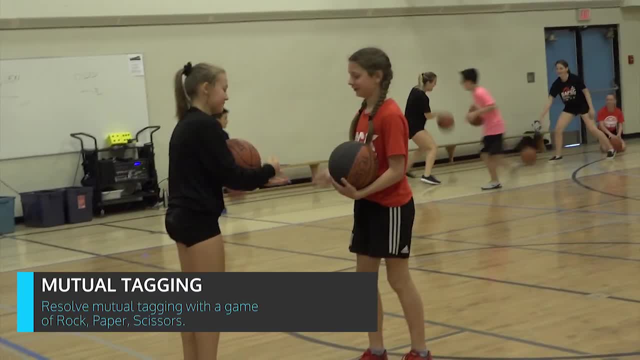 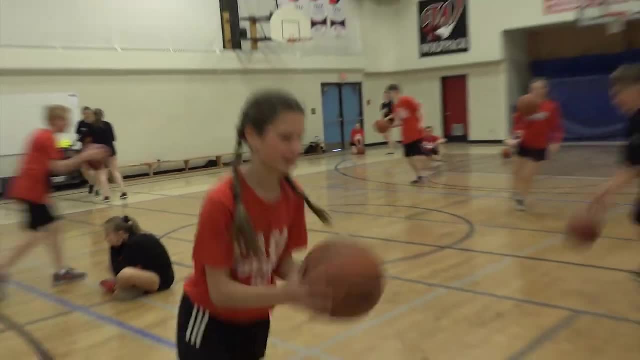 Pretty simple. Now, one item that comes up is what we call mutual. It's when two people tag each other at the same time. When that happens, you can do a rock, paper scissors. Whoever wins that stays alive, The other person sits down Freeze. 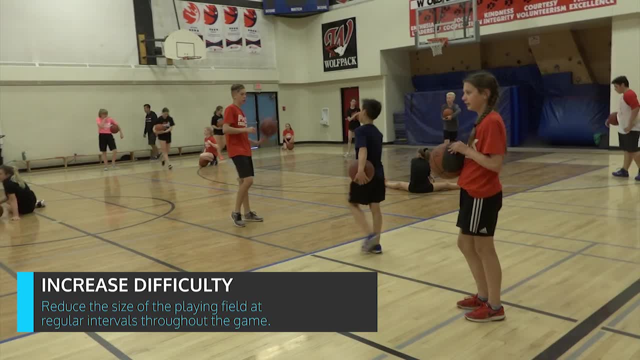 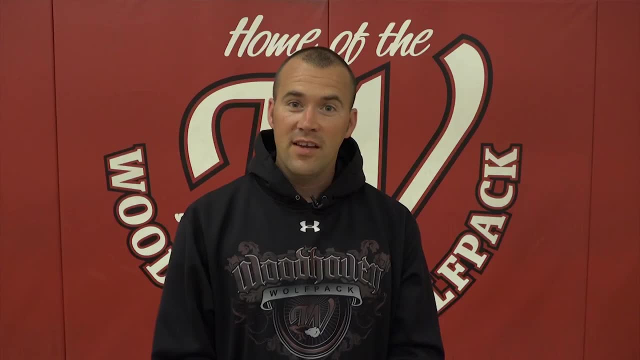 This time we're going to shrink the space only inside the main volleyball court, So that's inside the blue line With the dark hardwood. This game really doesn't come to an end. It's usually continual. It can come to an end if one person is left remaining. The teacher usually can yell jailbreak. 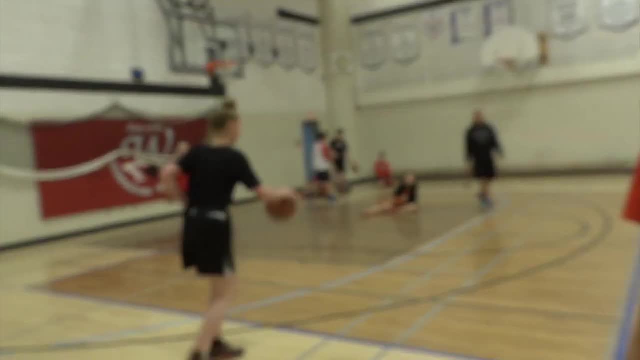 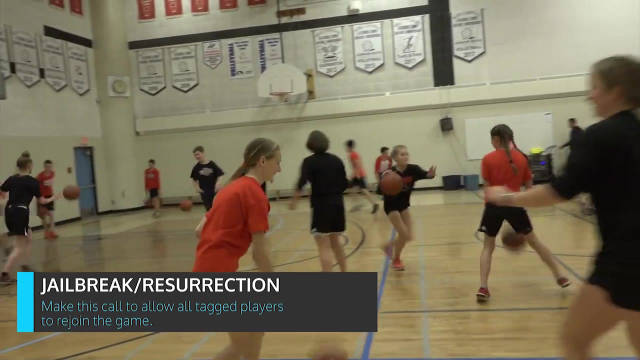 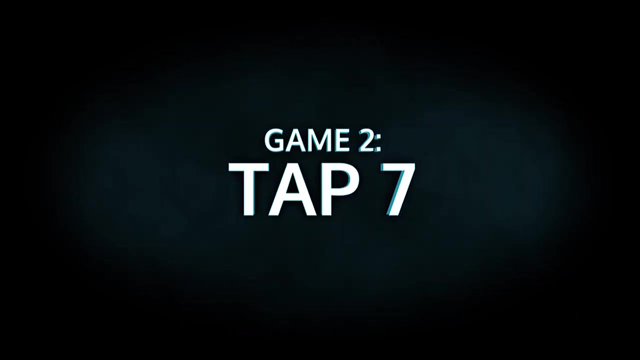 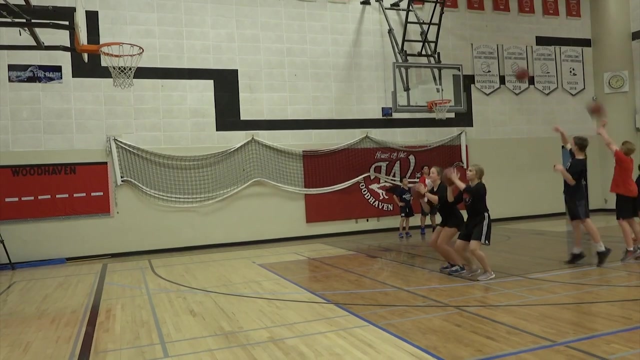 whenever they choose, trying to keep as many people back in the game working on their dribbling skills. Resurrection: Keep that head up, Keep moving, Keep moving. The next game we're going to explain is tap seven In order to play this game. 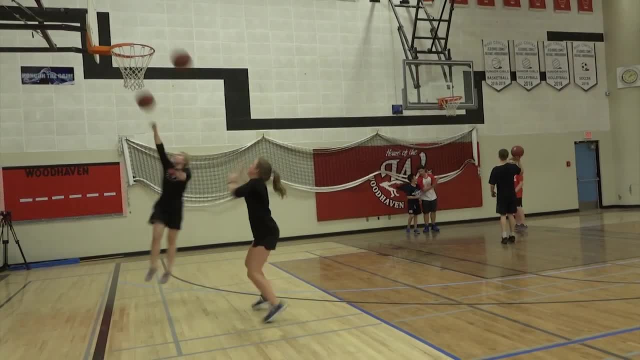 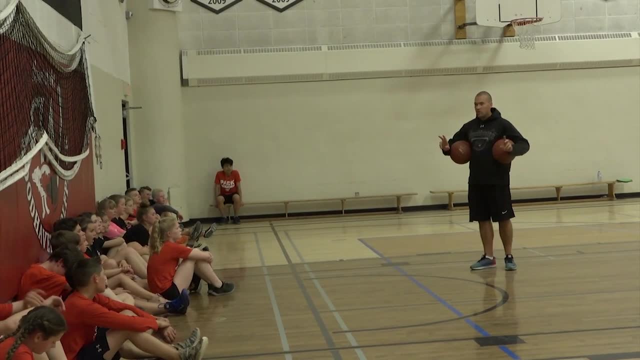 you just need to have two students or more. You'll need basketballs- one for every player- and nets to shoot on. So at your basket there'll be two shooters shooting. The game is called tap seven because you're going up to seven points. If we said tap five, the game would go to five Tap. 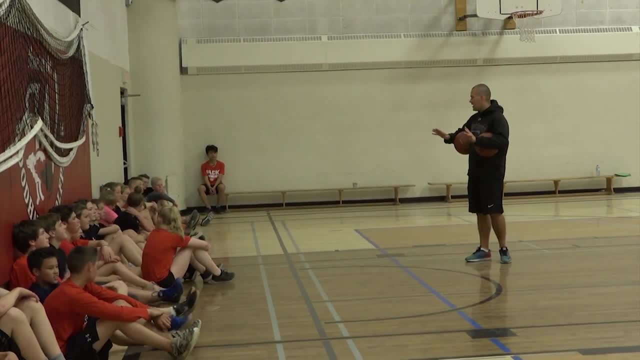 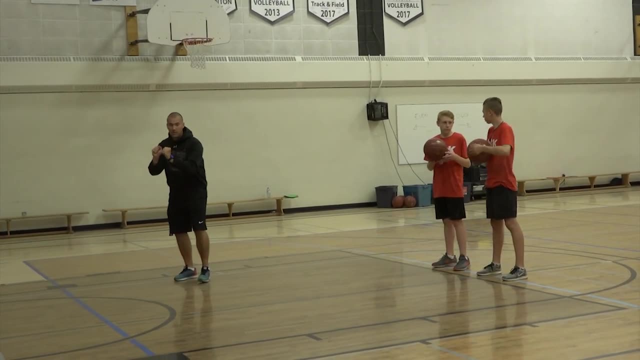 nine. the game would go to nine, But for today we're going to say tap seven. We got two shooters. Each has a basketball. When the game starts independently, they do it together. So all their basketballs, they tap them together. 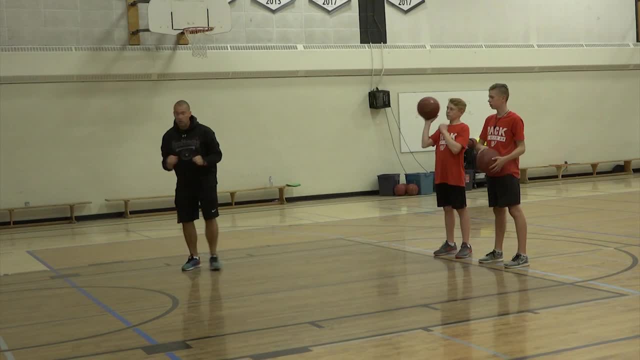 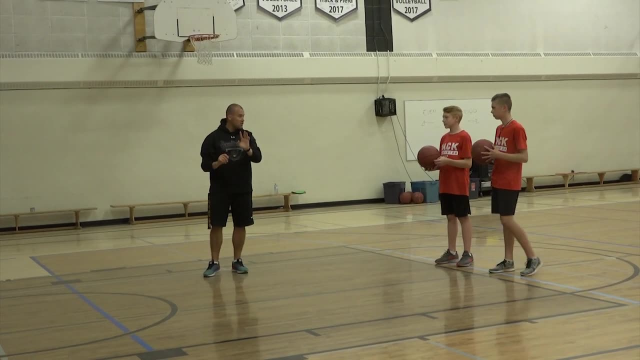 When that happens, that gives them free reign to shoot. If you shoot your first shot from the foul line, that's where you should start. If it goes in, it's two points. If you miss, you follow your shot to get your rebound. Once you put that rebound in, it's worth one point. But it is a race to see. 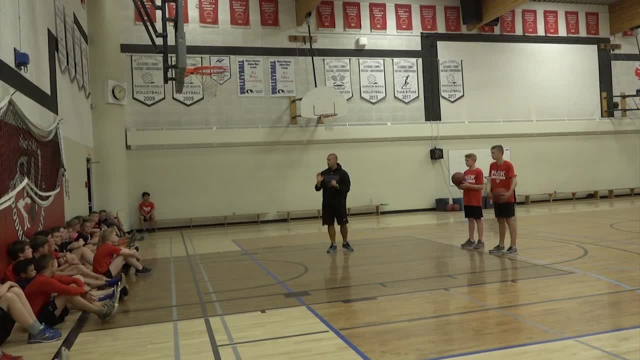 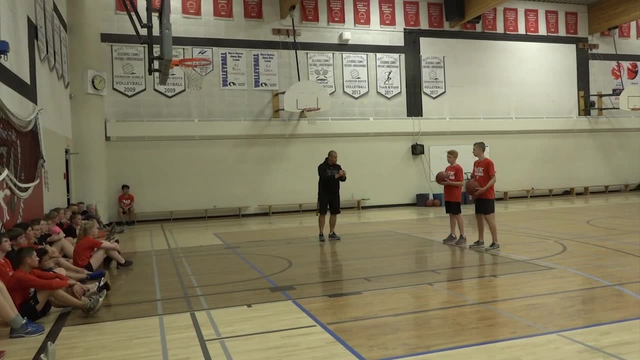 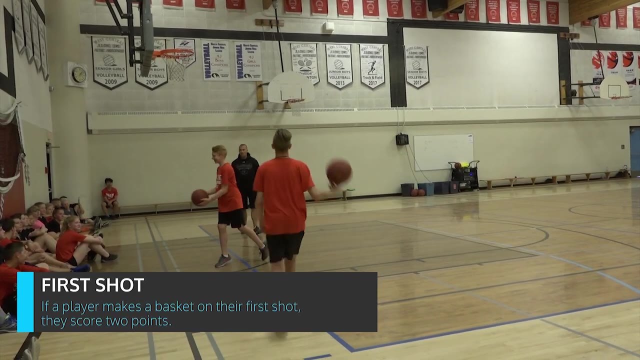 which of the two shooters scores first in order to earn the points. Any questions? So you guys are going to demonstrate. When you're ready, tap your balls together and do your first shot. Go ahead. Okay, Two points are scored there. They reset now. So the score right now is Austin two, Robert zero. 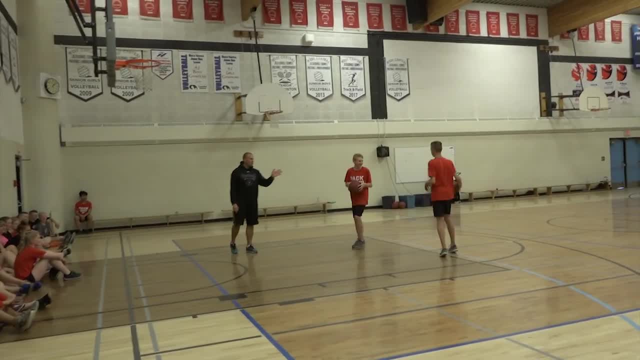 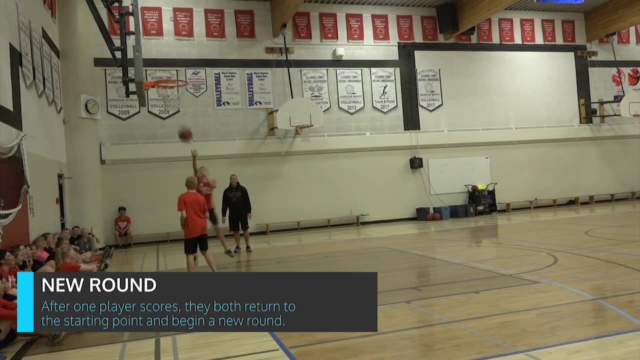 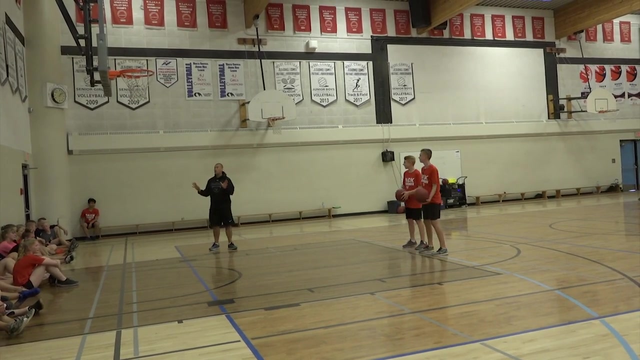 All right, Austin's on fire. Four nothing, Okay, Okay, Battle. Austin got the roll. Six, nothing, Six, nothing on this. So remember, game goes to seven. If you score over seven, that's okay. If he gets this in, he'd win the round. 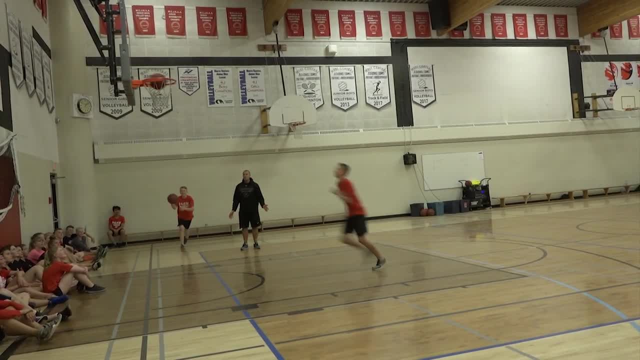 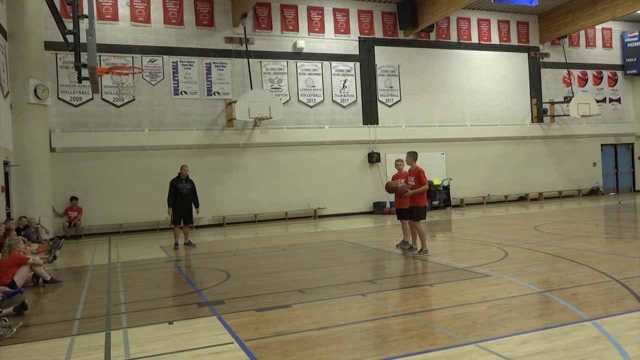 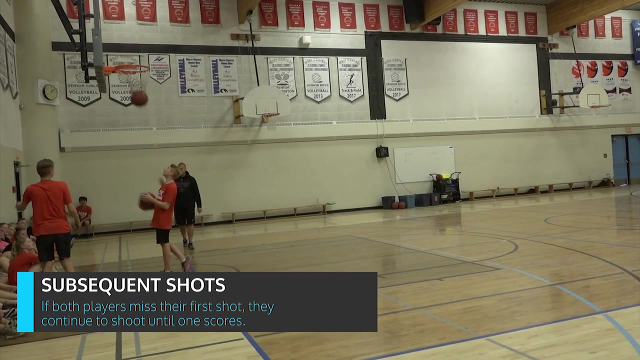 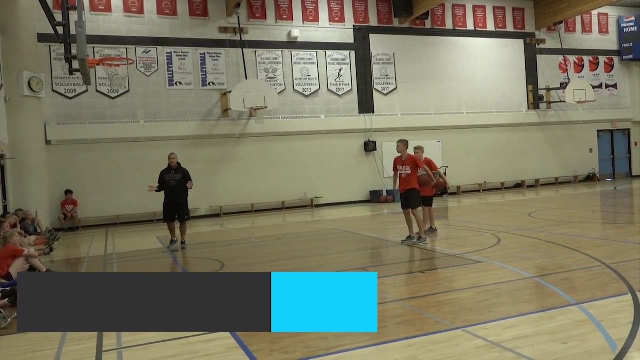 Come on, Robert. Come on Robert. Okay, What's the score guys? Austin six, Robert two. Okay. So on the missed shot there, both followed their shot. Austin scored. He would win seven to two that round. So now for our game. for the team version of this say: you two stay there. 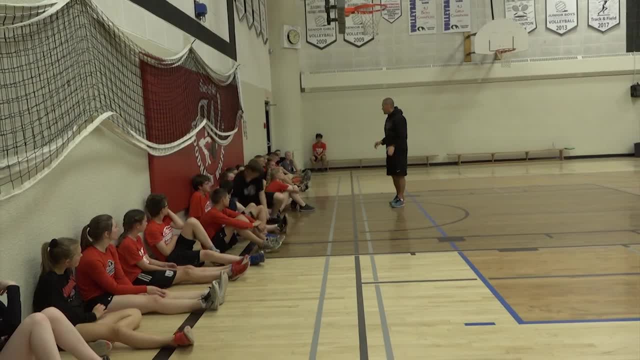 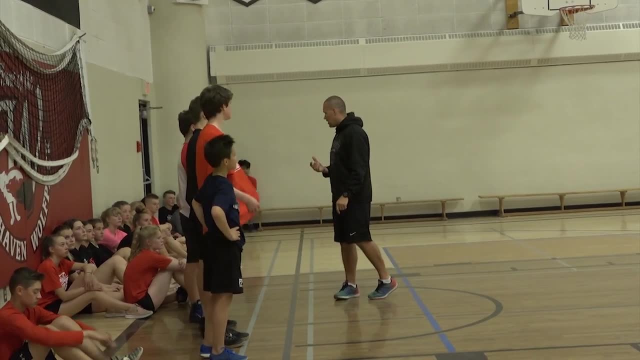 Can you guys stand up, One, two, three, four, stand up right here So say: these guys are on the same basket. They'll be underneath making a nice line. So just next guy in. So winner would stay, loser would rotate in. Does that make sense? So, Cruz, you're in there. Robert will be out. 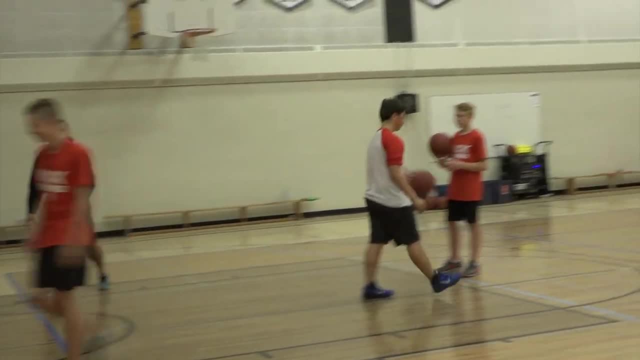 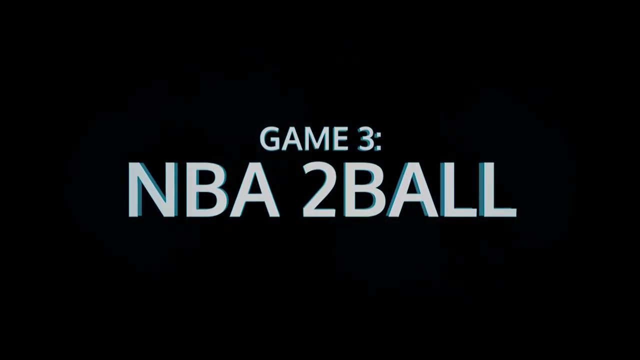 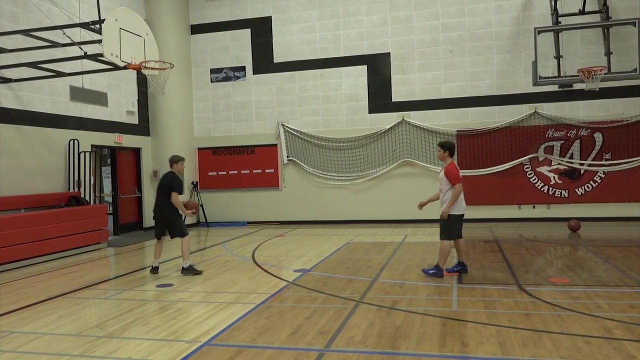 You play tap seven to work on your basketball skills while having a whole lot of fun. The next game we're going to show you is called NBA Two Ball. This game is a basketball shooting game done in partners. It is a great game for grades five to nine And, once again, 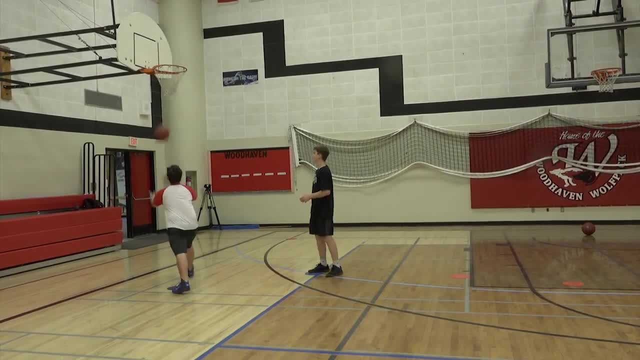 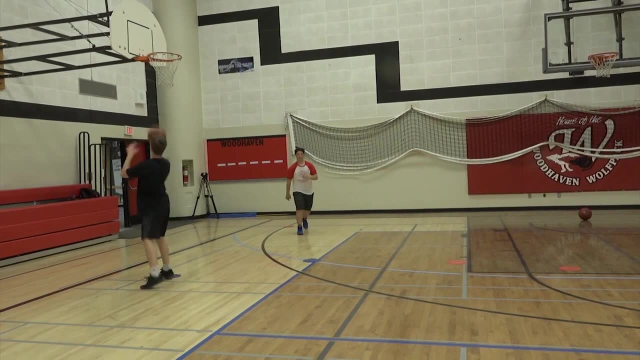 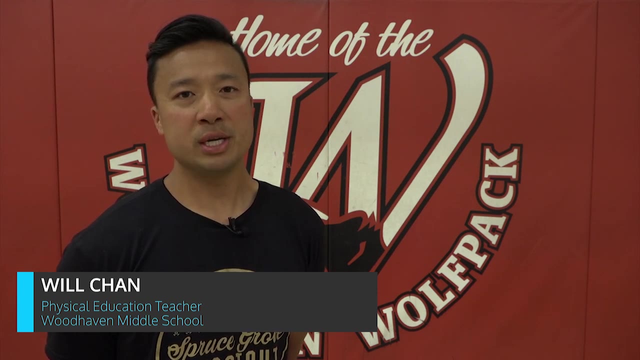 it can be modified up to grade 12.. The equipment needed are poly spots, as well as the music in the background. The two players are a team and their points are scored together. We teach this game to work on the kids: passing skills, shooting skills and cooperation. The objective of the game. 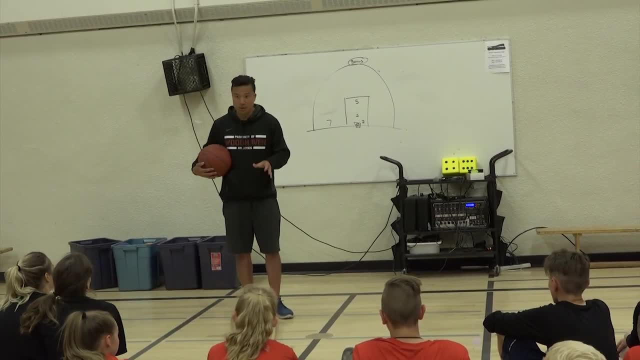 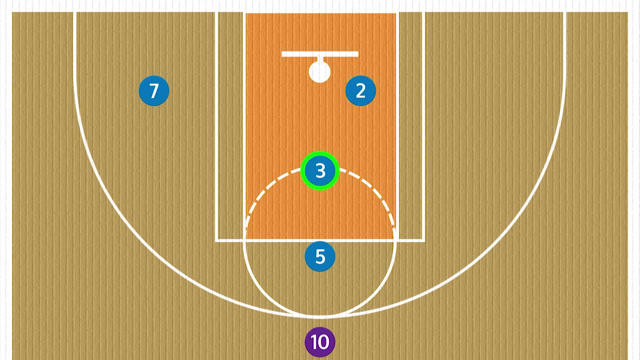 is to score as many points as you can with you and your partner. Here's a scoring grid: You get two points from this poly spot, three points from this one, five points, seven points. You take a bonus shot at the beginning of the game. These are the rules. 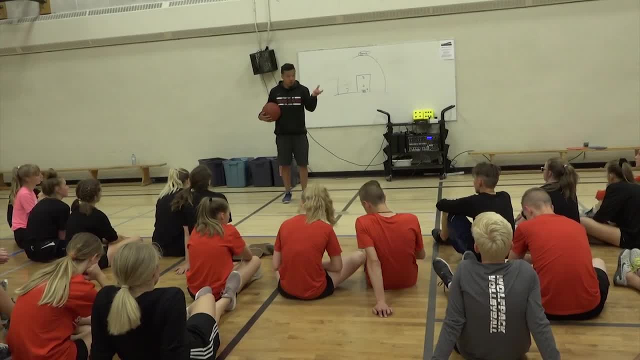 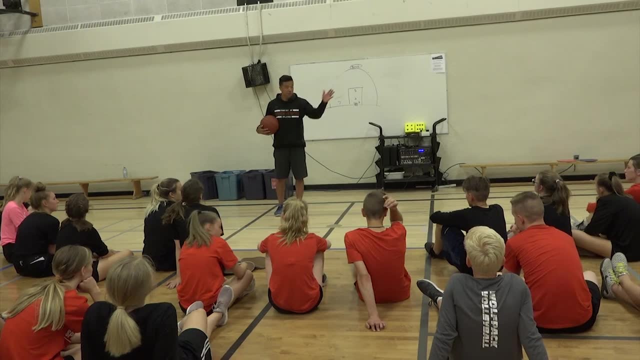 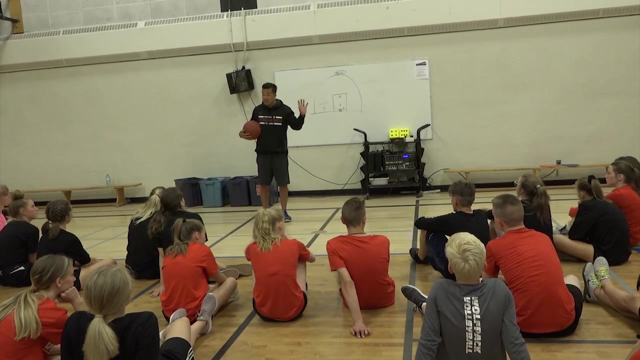 you cannot shoot twice in a row. You have to alternate shots and you cannot shoot from the same spot twice in a row. For example, if Koji shot from two, Caitlin cannot shoot from two Again. she has to shoot from another spot. So you have to keep on switching spots and taking. 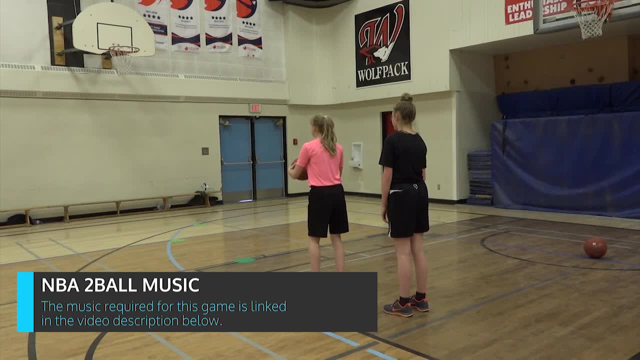 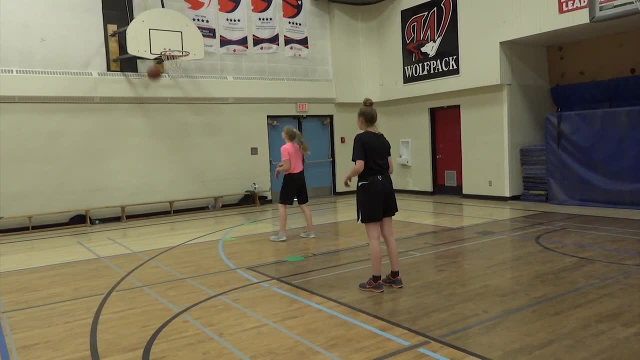 turns shooting. There was music to this game. How it goes it starts off with: this is Gatorade NBA Two Ball And you get 10 seconds for your bonus shots. Your bonus shots are worth 10 points. You get one each. 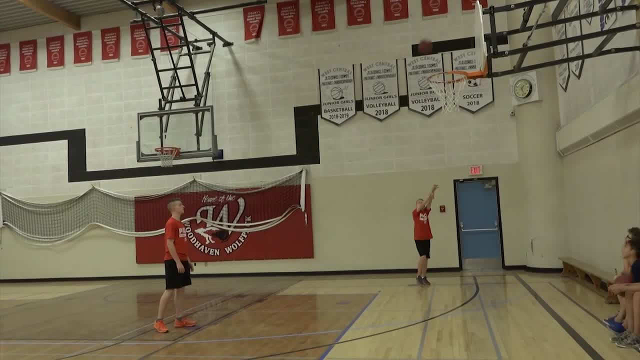 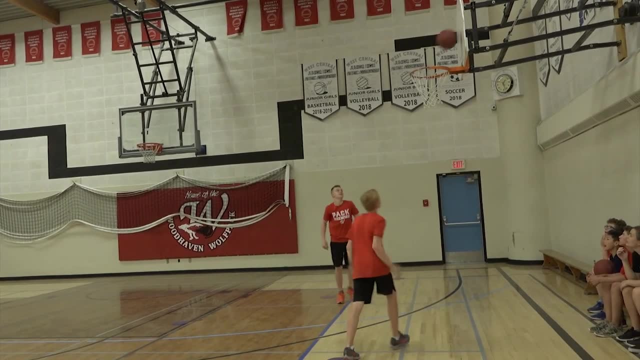 And then it'll start counting you down. You get a minute to score as many points as you can. If you're waiting underneath the basket, please count for the people shooting, because then they'll do it for you. after, Get ready for the bonus round. Get set. 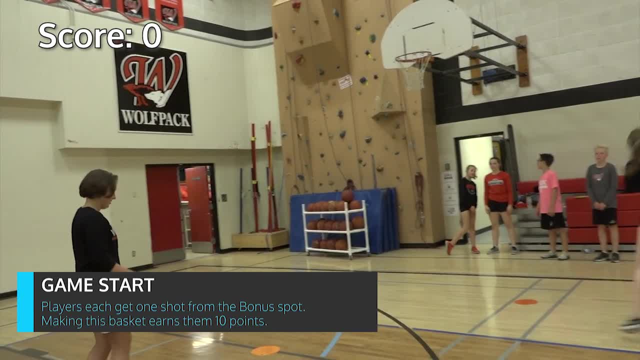 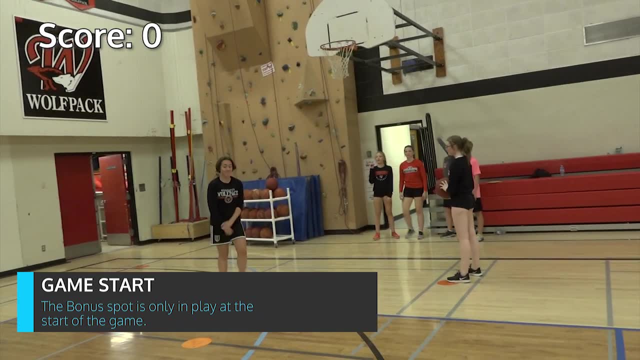 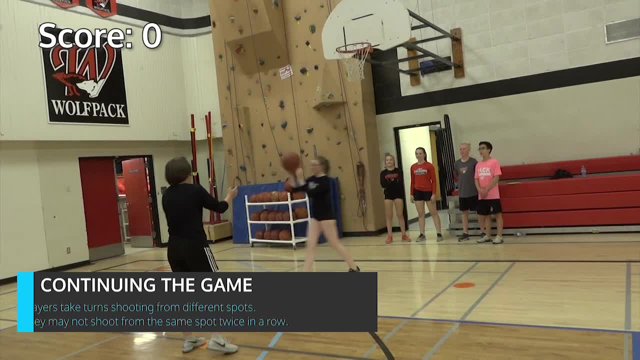 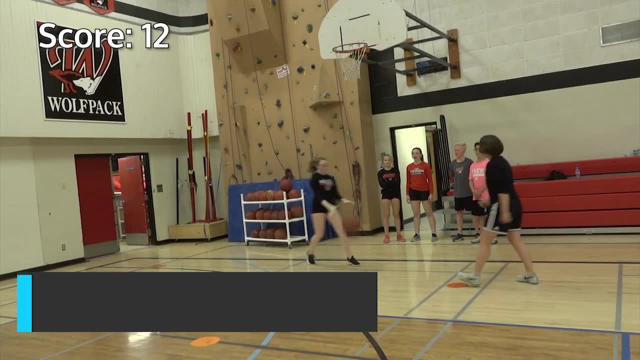 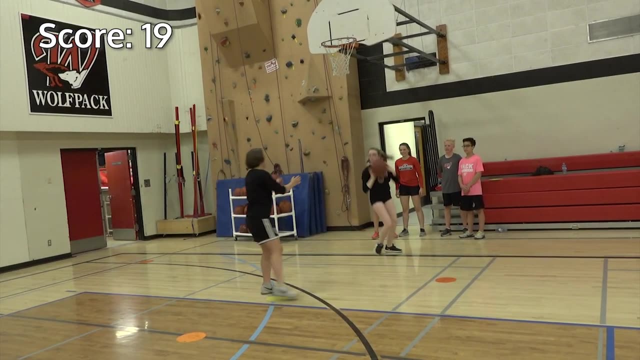 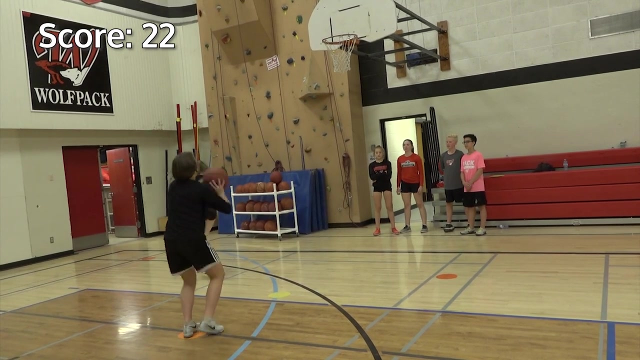 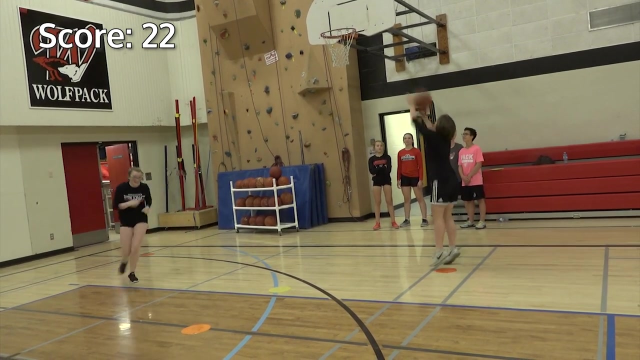 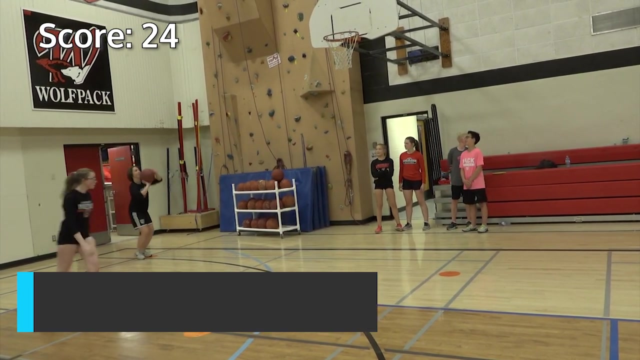 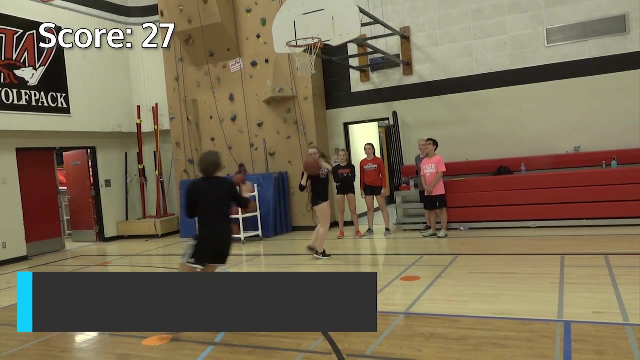 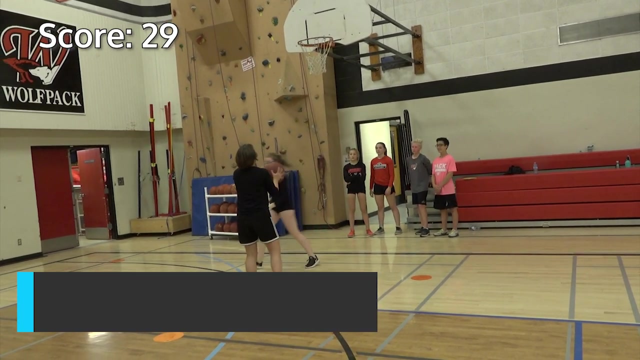 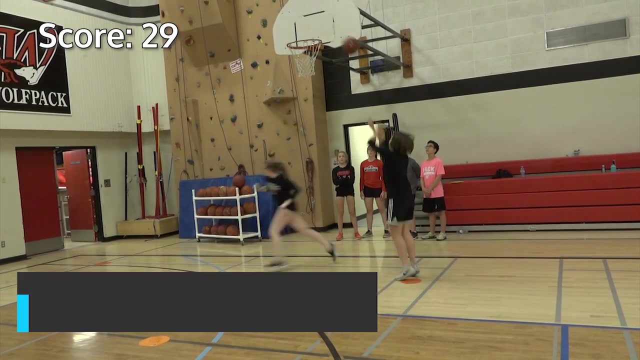 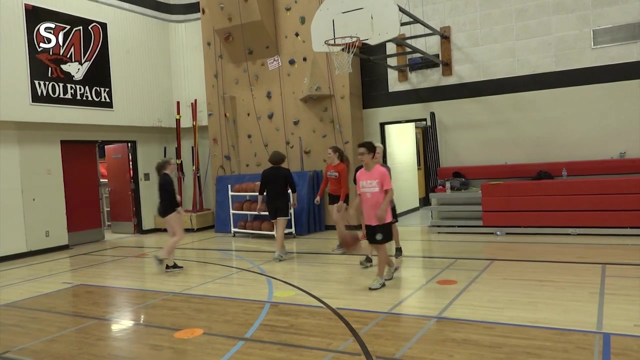 Five, four, three, two, one go. We'll be right back. All right, next group, Next group's up. If you wanted to, at the end of the minute you can get all the groups to come up. 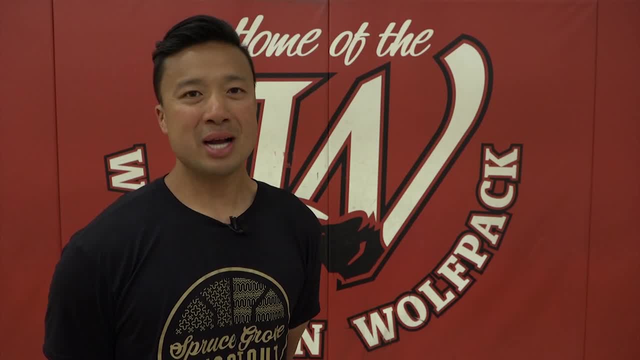 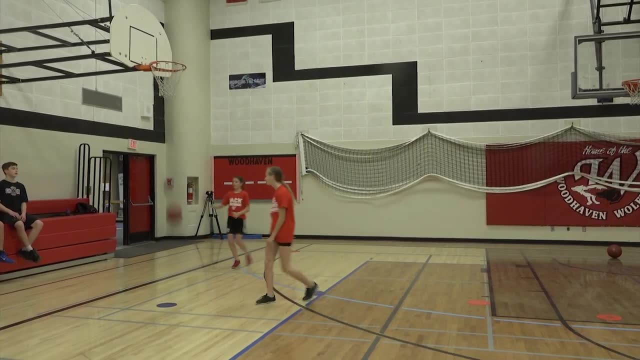 and tell you their score, What we do in our class. we track them all. At the end of the class we sit down and we go through all the scores and ask them what they can improve on next time. All right, next group. 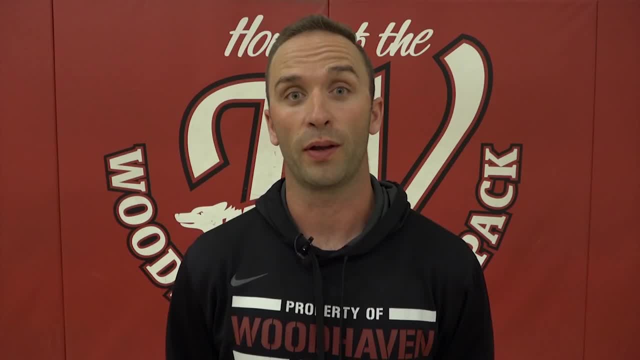 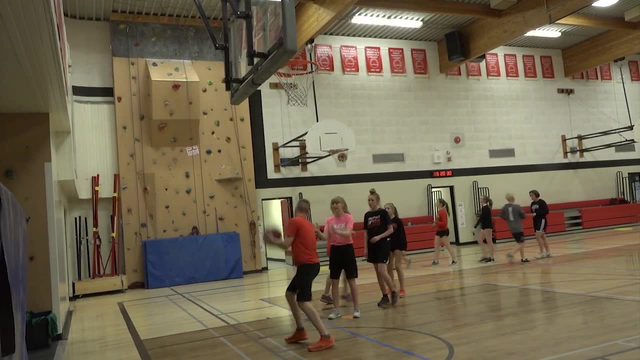 So the next game we're going to play is basketball bowling. Now, this game can be played ideally with 25, close to even 50- students in the gym at a time. It all kind of depends on the number of basketball nets. 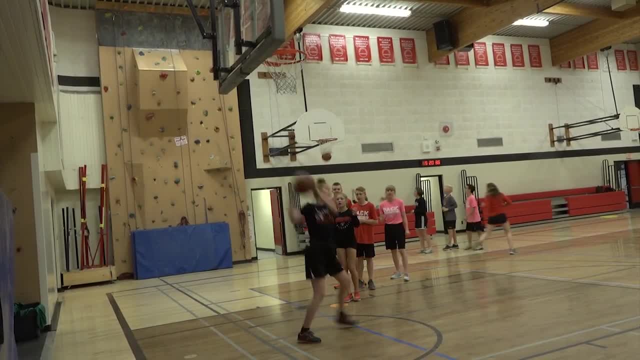 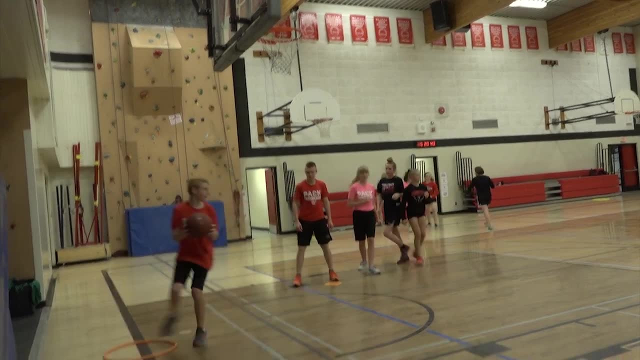 that you have available. Ideally we like to have students in groups of four to six and one group at each basketball net, But if we have larger groups then you can put two groups at each basketball net. We do this activity with students grades five to nine. 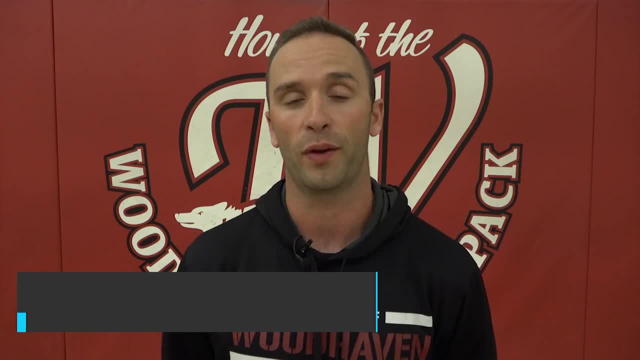 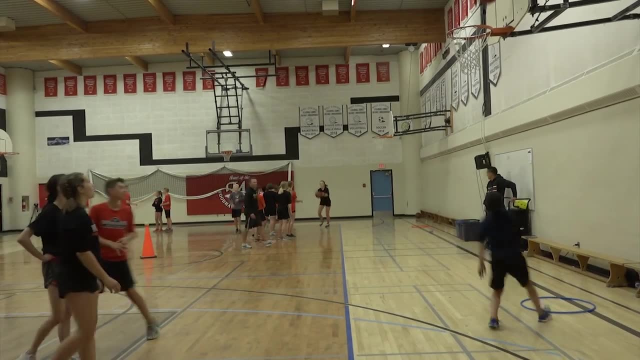 But again, it can be played and it could be modified for students as young as kindergarten all the way up to grade 12.. The equipment we need to play this game is one basketball per group, one hula hoop per group and one poly spot per group. 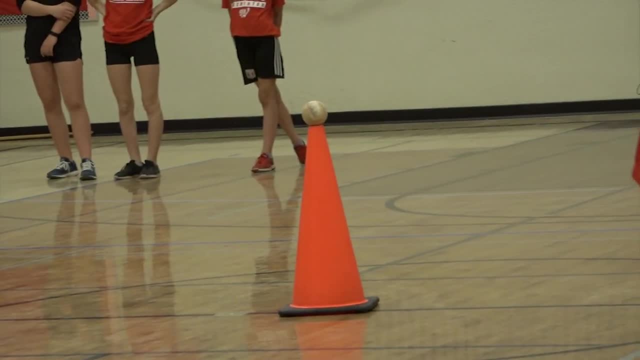 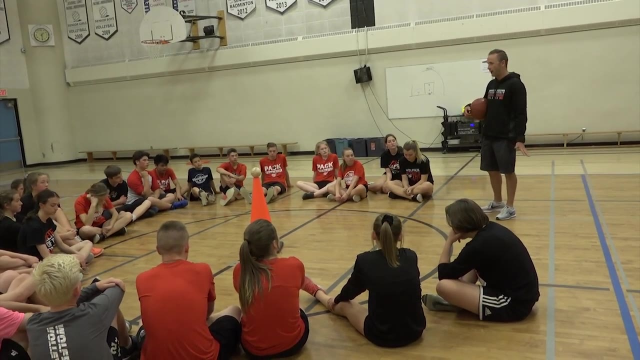 You also need a large pylon in the center of the gym with some type of ball to put on top. We just use a baseball or a softball. We're going to be split into groups of four to five students, right? So four or five. 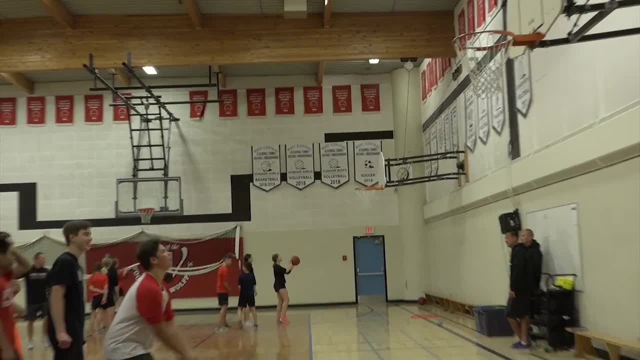 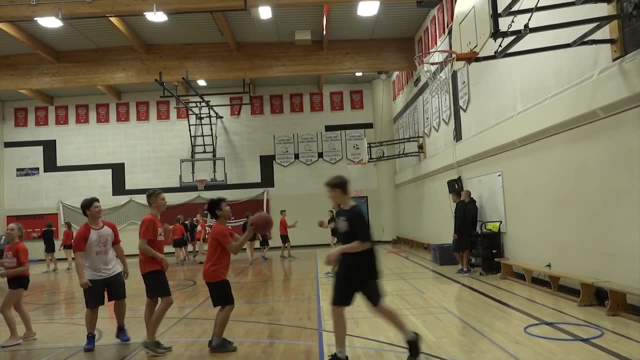 And each group's basically just going to be at one of the six baskets. right, There's going to be a poly spot at each basket or the basket you're assigned to right To start off with. you're just going to line up behind that poly spot.